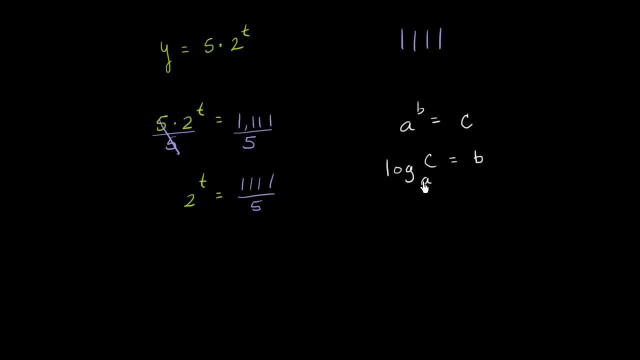 a to the b power is equal to c. Log base a of c is equal to b. Log base a of c says: what power do I need to raise a to to get to c? Well, I need to raise a to the b power to get to c. 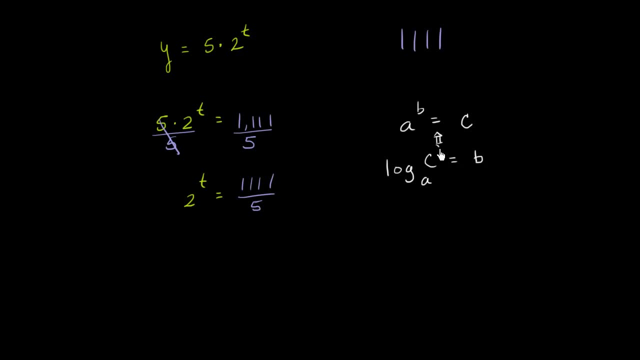 a to the b power is equal to c, So these two are actually equivalent statements. So let's take log base 2 of both sides of this equation. So on the left-hand side you have log base 2 of 2 to the t power. 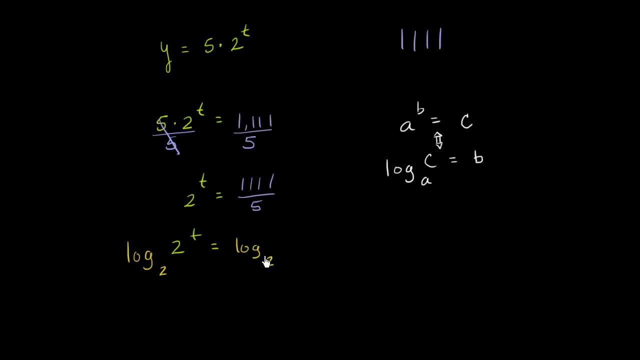 And on the right-hand side you have log base 2 of 1,111 over 5.. Now, why is this useful right over here? So this is: what power do we have to raise 2 to to get to the 2 to the t power? 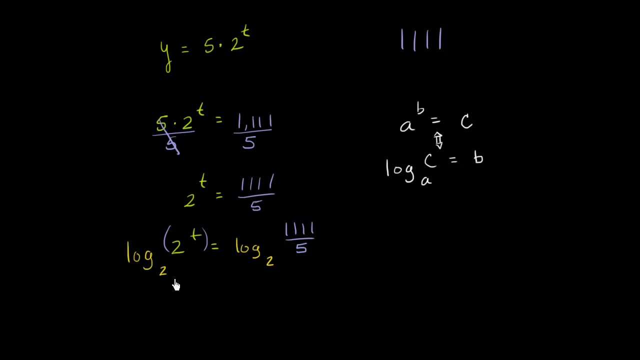 Well, to get to 2 to the t power, we have to raise 2 to the t power. So this thing right over here just simplifies to t, That just simplifies to t. And on the right-hand side we have 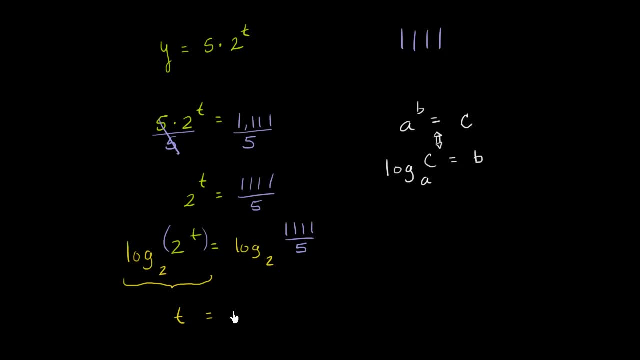 log base 2.. We have all of this business right over here, So I'll just write it over. t is equal to log base 2 of 1,111 over 5.. So this is an expression that gives us our t value. 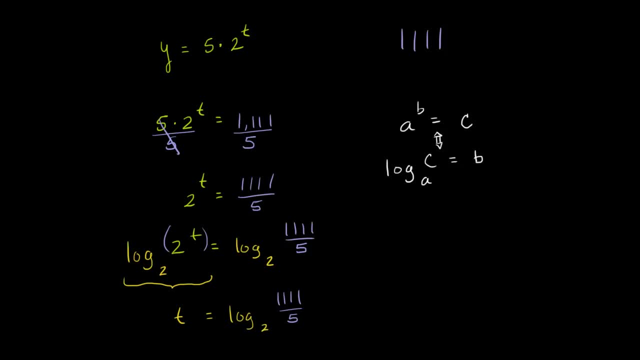 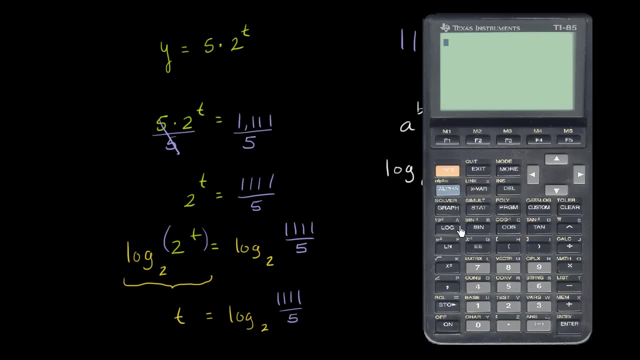 But then the next question is: well, how do we actually figure out what this is? And if you take out your calculator, you'll quickly notice that there is no log base 2 button. So how do we actually compute it? And here we just have to apply a very useful property. 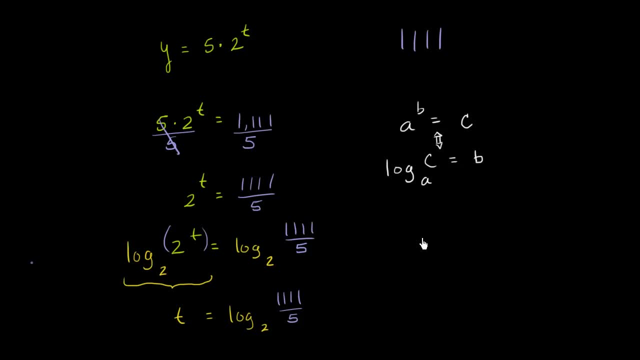 of exponents. If we have log base 2 of- well, really anything. Well, let me write it this way: If we have log base a of c, we can compute this as log base- anything of c over log base that same, anything of a. 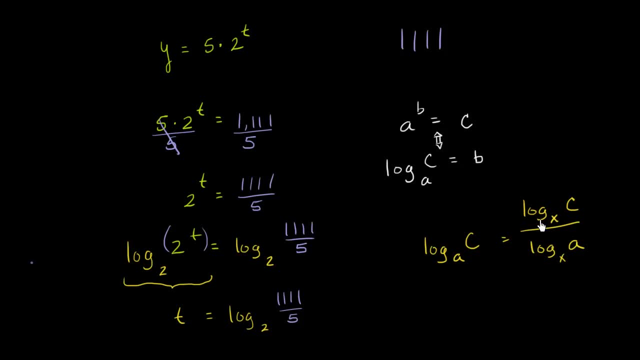 This. anything has to be the same thing. OK, And our calculator is useful because it has the log. When you just press log, it's log base 10.. If you press ln, it's natural log or log base e. I like to just use the log base 10..